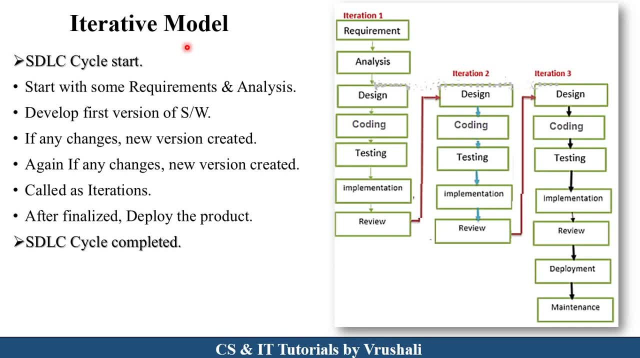 Now the first thing is what exactly iterative model See here in this particular diagram? This is a structure of iterative model. As we know, every software development lifecycle start with the requirement and analysis phase. There is a project analyst who collect the requirement from the customer and analyze those requirement. This is the first phase in software development lifecycle. Correct Now, after collecting requirement, they design the particular product. after that coding and after that testing. Now completing this implementation in iterative model. 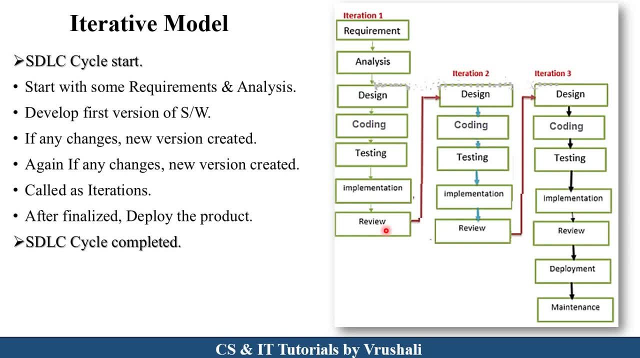 Then they review the product. Okay, Review the product means if customer want any new changes or if there are any new versions or if there are any new features, So this thing are available. Then they review the product and again perform the design coding testing in next iteration. Okay. So they again perform design coding testing and again review this complete implementation. Again check if there are any new iteration, new versions are there. 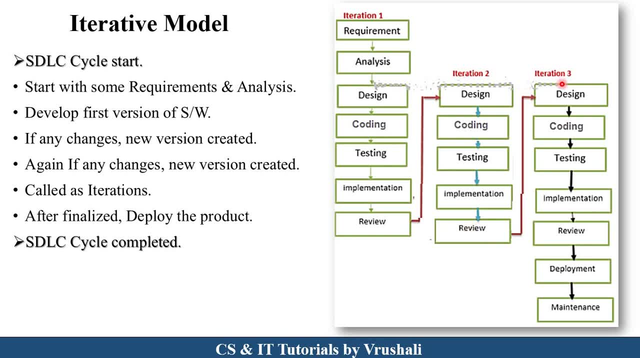 If it is available there again move to next iteration. Then they again design the product, again perform coding testing and again review this complete implementation. Now again they check if any new changes, new versions is there. If not, then they deploy the product in customer and maintenance a particular customer product. So this is called as iterative model. So simply means iterative model. You can develop a product in multiple ways. 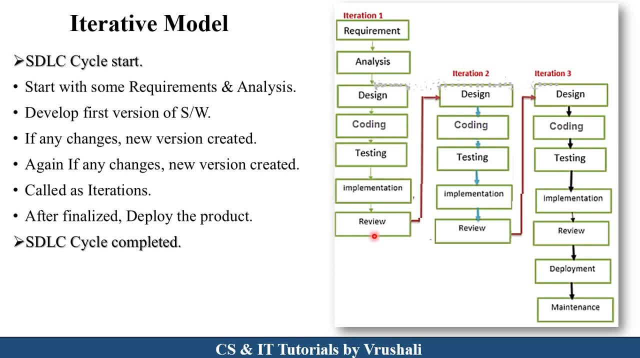 multiple iterations. ok, here customer requirements are not fixed as per waterfall model. customer requirements are continuously change, or new updates, new versions are there, right, so you can made a product as per the new iteration, as per the new features clear. let's take one example like whatsapp. when there are whatsapp, updates are available, so there are some new. 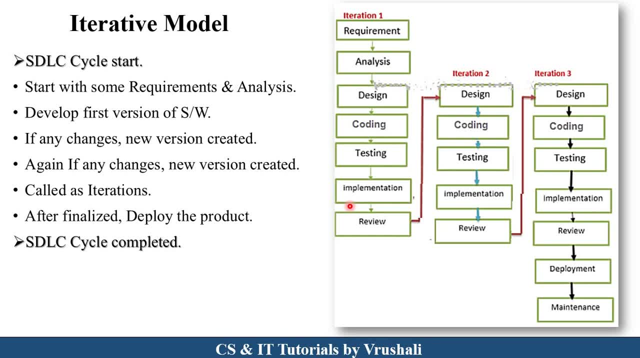 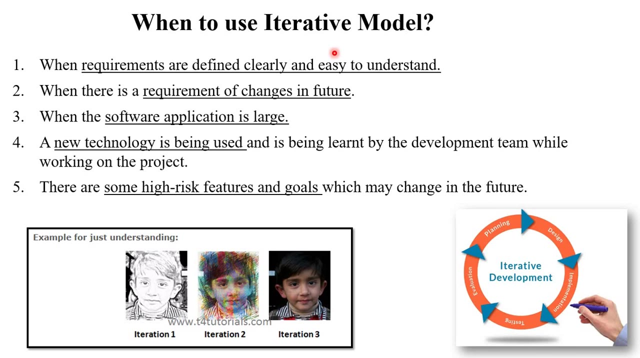 features are there, right. so again you update your whatsapp again after some months. there are again some new features. you update your whatsapp from google play store, so again there are some new features are available, right. so this same thing. have updated in iterative model- clear. next, now the important thing is when to use iterative model. so in iterative 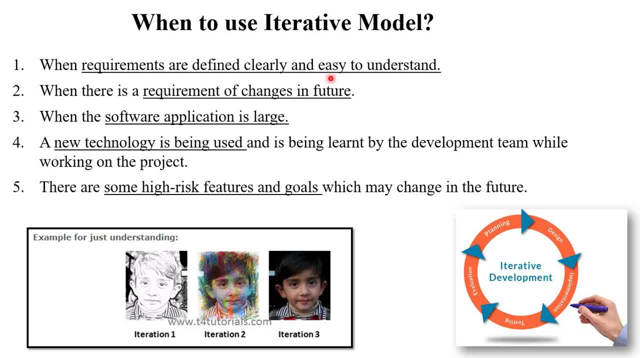 model requirements are clearly and easy to understand because requirements are changes or requirements are not fixed. in waterfall model requirements are fixed from the customer but here iterative model requirements are not fixed. you can change the requirements in any phases of particular iterative model. here this iterative model generally used when there is a large software application. large project is there in this. 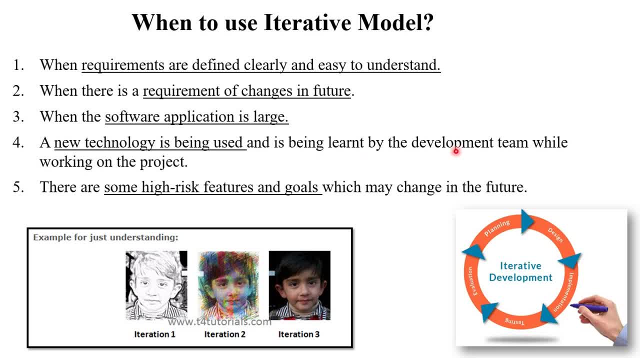 iterative model. new technologies are used, so every developer or every programmer they need to learn new technology because each iteration new feature is there, so you need to apply some new technology. new frameworks are there and if there are some high risk features in there, in particular iterative model, so that will be change in. 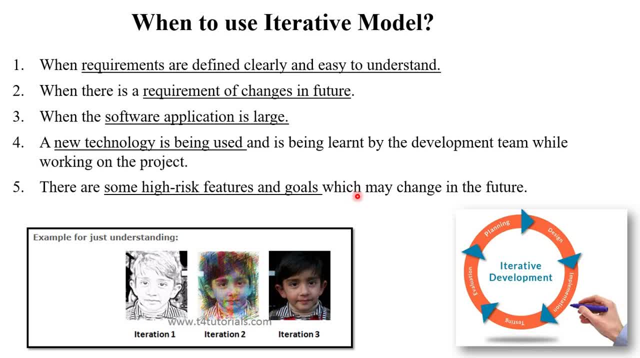 future means in iteration one, if there are any errors or if there are any new updates are not available, so you can move to iteration two, then again you can move to iteration three in this way clear. so in this only particular requirements iterative models have used. let's see here in this example: this is a just. 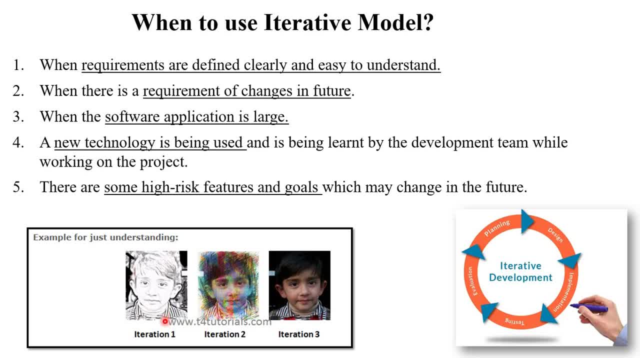 example for understanding, see here this image for iteration one. but this image not having that much accuracy or colors representation, so it moved to iteration two. again this image again not have any particular accuracy, then they again move to iteration 3.. now in iteration 3 there is a 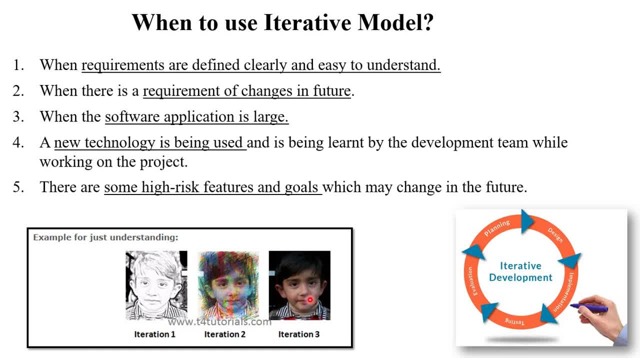 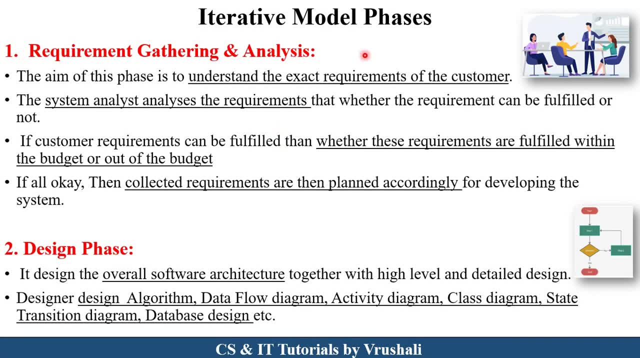 accuracy and colors in particular, image right. so this is a last product, clear. next, now again iterative model phases. we already discussed these phases in software development life cycle in detail. the first phase is requirement gathering and analysis. here the particular project analysts gather all the requirements from the customer. there is a communication. 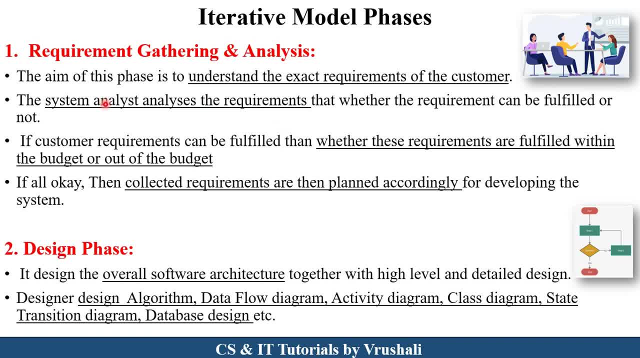 between customers and project team. now system analyst analyze those requirements: if a particular requirements can be fulfilled or not by the project team, or if the particular requirements within the budget or out of budget. so they analyze all those things. if all, okay, then they collected all the requirements and plan your complete project. they decide the starting of project and 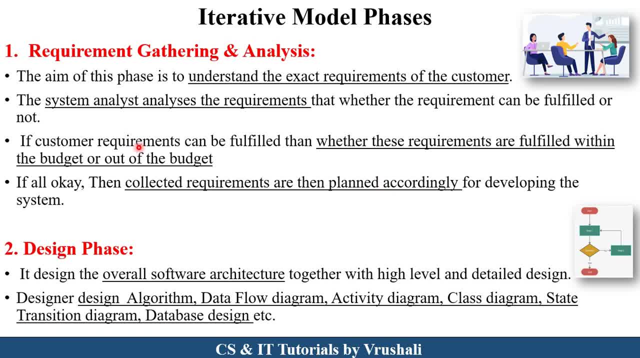 different phases of the project. now, after collecting requirement, the next phase is design phase. in design phase, overall software architecture have decided here ui ux designer design the product by using some algorithm: data flow diagram, activity diagram, class diagram, state transaction diagram and database design. here design represent how your product look like in 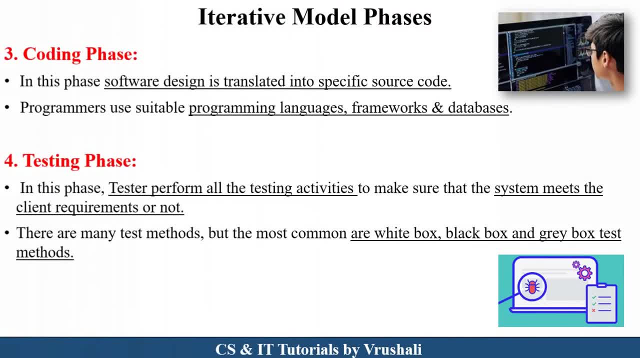 future. next now, the next one is coding phase after designing. so there is a coding phase. so programmer or developer converts the product to a software and then the next phase is design phase in design, software design into the specific code. for that purpose they use different programming languages. 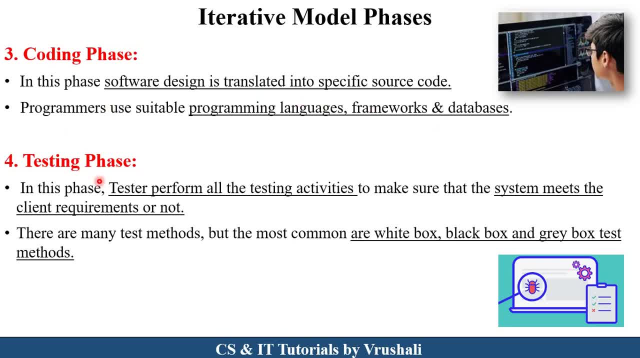 framework or databases. after coding, the next part is testing phase. here tester perform different testing activities and check that your product is meet to the customer requirement or not. so they perform different testing methods, like white box, black box, gray box, testing as per, suitable for the particular project. next, 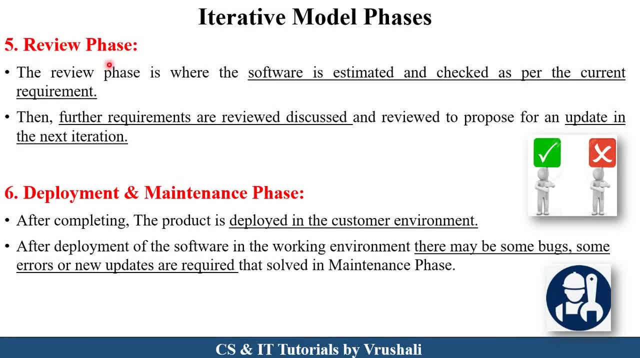 now, after testing, there is a review phase. in each iteration there is a review phase. so review phase means here the particular reviewer check that the particular software is as per the customer requirement or not, or if customer want any new requirement or new features in particular project or not. so reviewer check this thing. if customer want new project, then they move to next iteration. 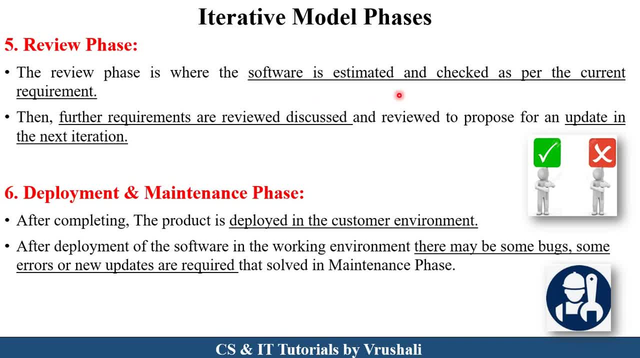 and they perform again design testing, design coding and testing and again review the product in this way. so every iteration there are new features, new updates are available now. last one is deployment and maintenance. so at the end the products have developed as per the customer requirement completely. so last phase is deployment phase. 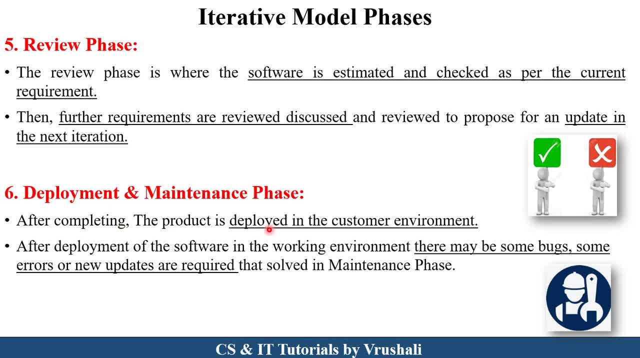 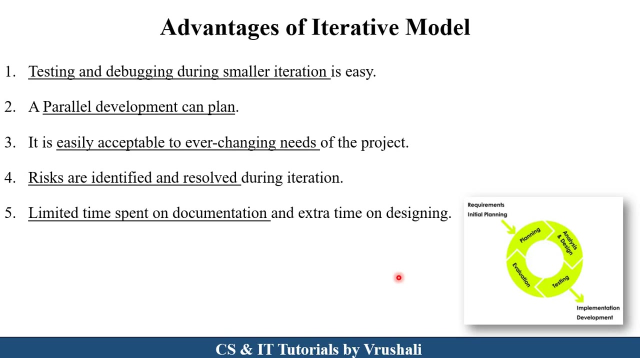 deployment means after completing the project, product is delivered to the customer or customer environment. and in maintenance phase, after deploying product to the customer and installation, if there are any bugs, there are any issue or customer want any new updates, so that this all things solve in maintenance phase. clear next. now the next point is advantages of iterative model. so the main advantages is testing and debugging done during small iterations, right, because every iteration they check any errors have not, then they move to next iteration. right, so parallel development can plan means there are multiple